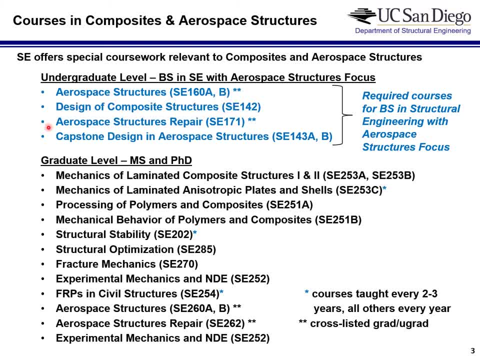 This is a two-quarter sequence And then, typically in your senior year, you take these courses. programs in the country do not do, uh, or i would say almost none of them do this class, but, um, we do. all students take composite structures, learn about composite materials. 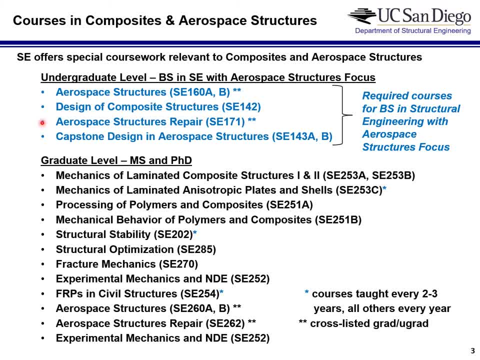 all students will take aerospace structures repair, which is really a course related to how do you join different portions of structure together using adhesive, bonding or or bolted assembly, how do you predict failure and design those efficiently. and then a very special course sequence we've created is the capstone design, and that's the set of two courses that you take. 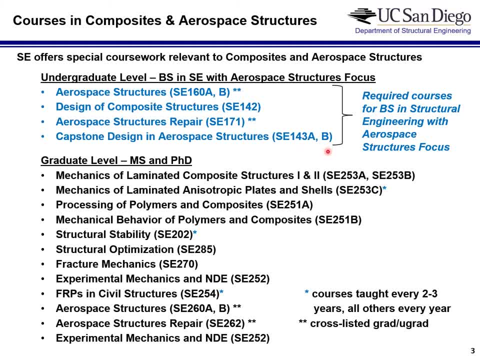 in your final year, and this is involving a design, build, testing of composite structures. so all students who are going to specialize in the aerospace focus sequence would take these courses. additionally, i've listed graduate courses here and these courses are available to be taken by undergraduates by petition, if you're performing well and you get permission from the instructor. 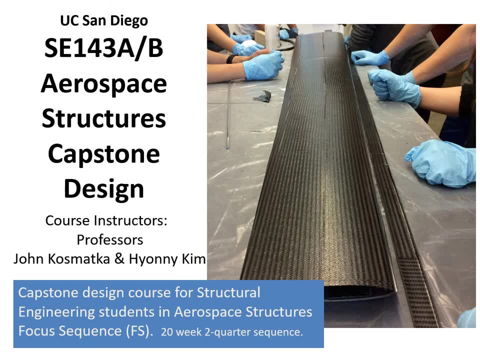 i'll talk a bit more about the capstone design course, and that's something that that we've put together that focuses on applying everything you've learned from the coursework as well as not just in the aerospace focus, but also including the core courses and and applying it into hands-on design, build and test, and we're 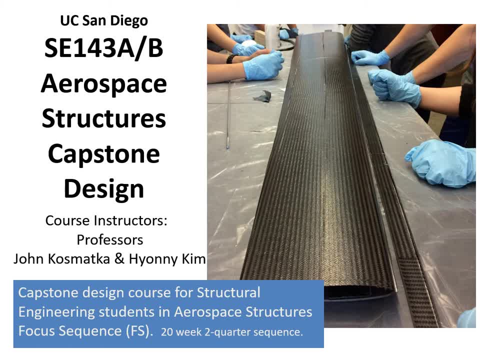 transitioning this even into fly. what we've been doing recently- and you know this could evolve in different timing, but we've been having students do- is design, build, test these unmanned aircraft wings. here's a photo of this and this is a. this is a two, two sequence. two-quarter sequence course. 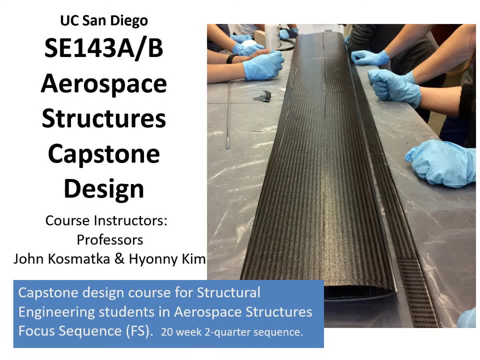 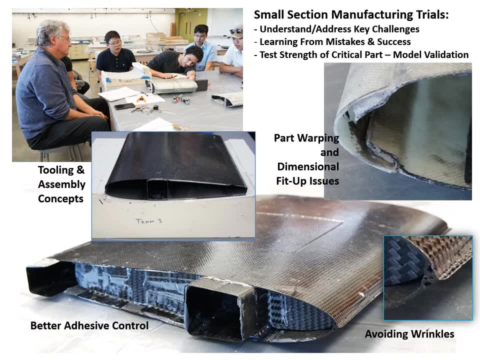 right? so basically 20 weeks of activity involved, right? so what makes this course very unique is the not only the rigorous analysis and engineering aspects, but also the hands-on nature of it, and we spend a lot of time in the first first part of the course just making things. 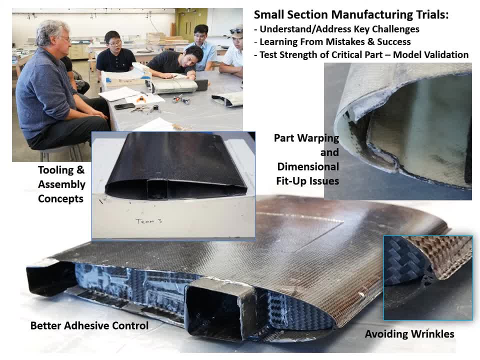 designing, making testing, and you know this set of photos actually shows failed parts or parts that have a lot of problems, and one of the important things that we always benefit from are making mistakes and learning from. you know how things don't fit up: getting flaws and wrinkles in the structure or using too much bonding. 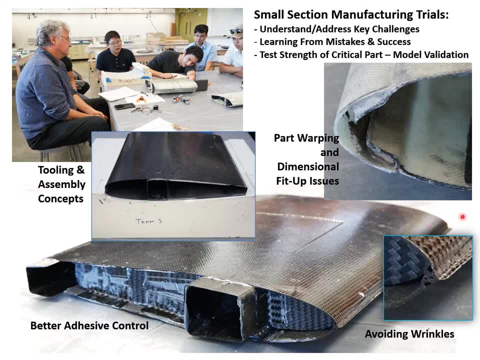 learning from these things, right? this is extremely important aspects of engineering. that's an important part of learning from these things, right? this is an extremely important aspects of engineering. that's an important part of this class. these are all, let's say, small section practice structures that this class. these are all, let's say, small section practice structures that 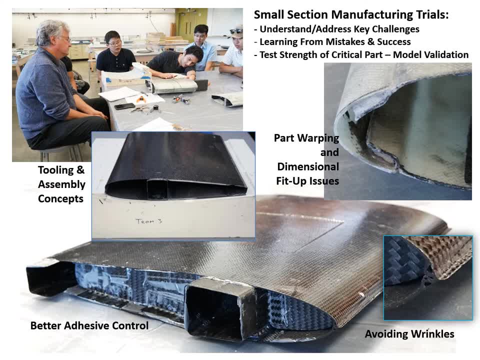 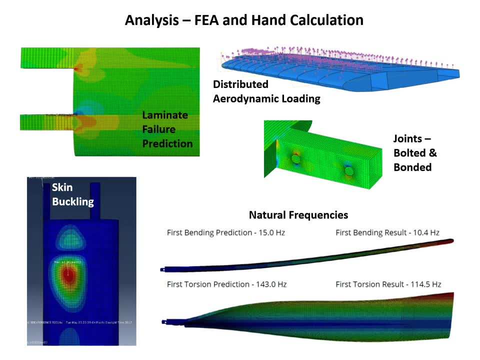 students have made to learn how to better make a larger size structure. students have made to learn how to better make a larger size structure. a major portion of this class is really on the design and analysis, and that's what makes us say bachelors of science in engineering, as opposed to something. 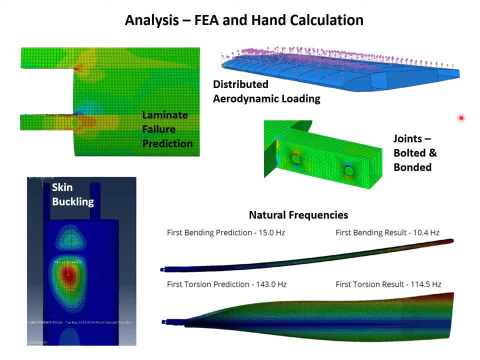 what makes us say bachelors of science in engineering, as opposed to something related to just putting something designing, related to just putting something designing, related to just putting something designing something you know and building something you know, and building something you know and building it without really understanding how it's. 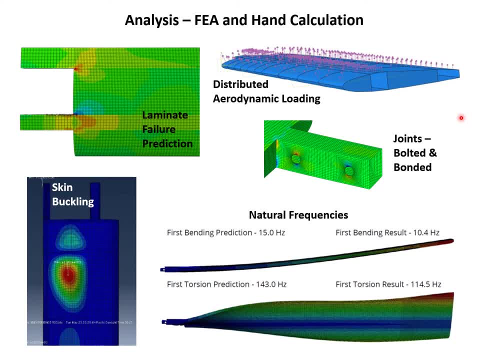 it without really understanding how it's it, without really understanding how it's gonna behave, and we spell spend a lot of gonna behave. and we spell spend a lot of gonna behave. and we spell, spend a lot of time focused on predicting the behavior, time focused on predicting the behavior. 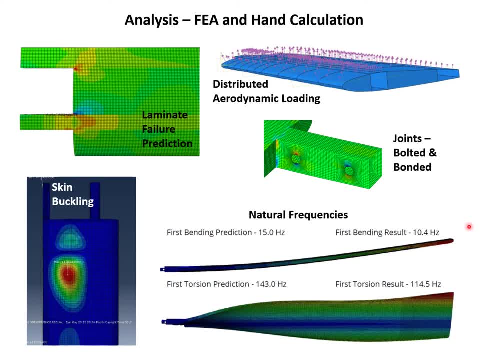 time focused on predicting the behavior using computer analysis as well as using computer analysis, as well as using computer analysis, as well as classical hand calculation analysis, to classical hand calculation analysis, to classical hand calculation analysis, to predict things like buckling of the skin. predict things like buckling of the skin. 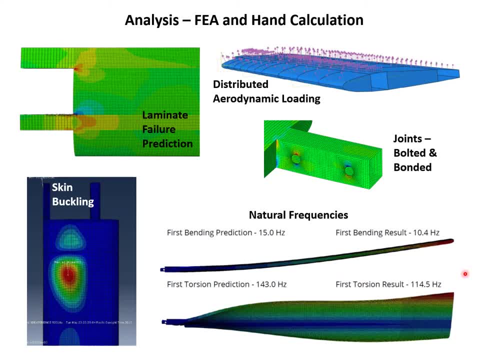 predict things like buckling of the skin and how much deflection or how much, and how much deflection, or how much deflection, or how much deflection, or how deflection, or how much deflection, or how much deflection, or how much vibration. what vibration? 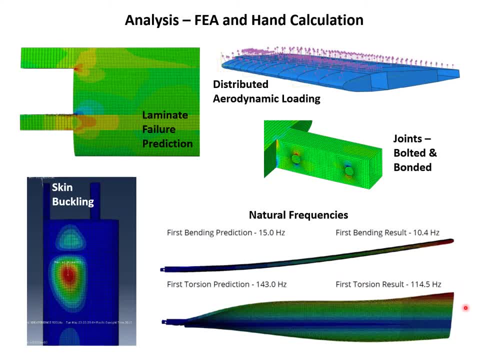 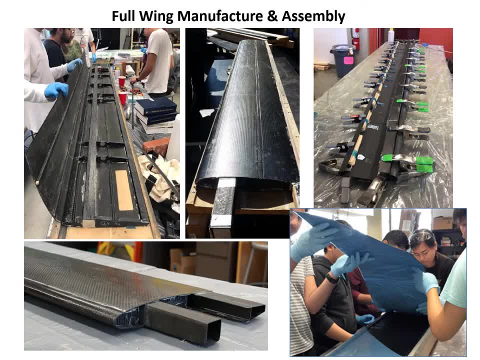 it, or when the composite laminates would it, or when the composite laminates would fail. another major portion of the class is another major portion of the class is another major portion of the class is this actual fabrication and assembly and this actual fabrication and assembly and this actual fabrication and assembly and learning how to create tooling to make. 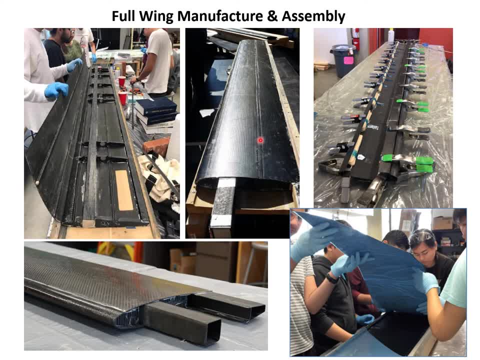 learning how to create tooling to make. learning how to create tooling to make these structures. learning how to put the these structures. learning how to put the these structures. learning how to put the structures together and achieve good structures together and achieve good structures together and achieve good quality. 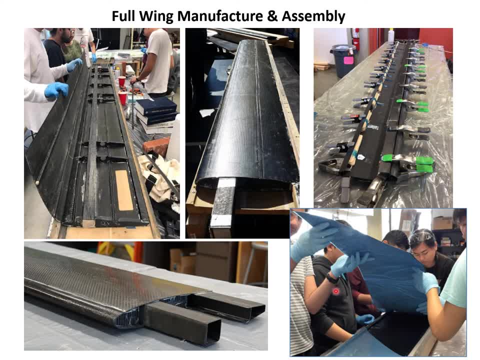 quality. quality achieve good fit up. some of the soft achieve good fit up. some of the soft achieve good fit up. some of the soft skills that are very important is skills that are very important. is skills that are very important is teamwork and how do you work with other. 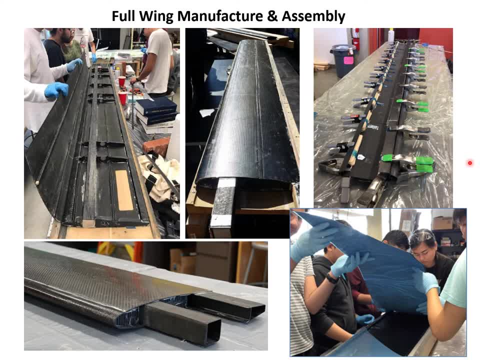 teamwork and how do you work with other teamwork and how do you work with other people. how do you be be productive as a people? how do you be be productive as a people, how do you be be productive as a team and make sure that things are team and make sure that things are? 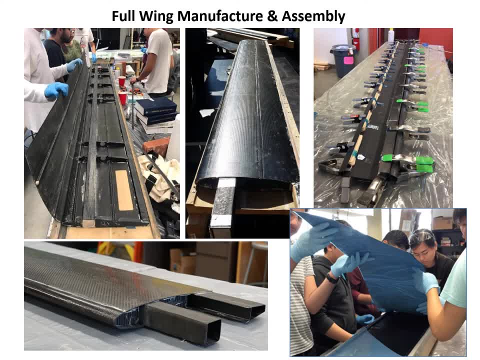 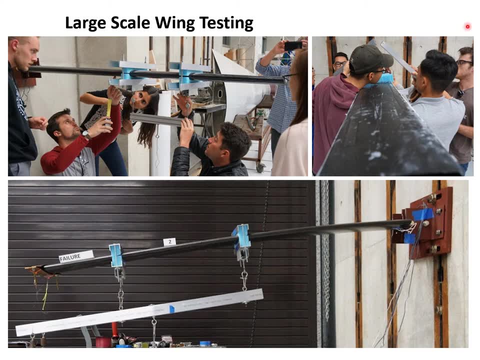 team and make sure that things are getting done as a team. that's how real getting done as a team. that's how real getting done as a team. that's how real world engineering is going to be. world engineering is going to be, world engineering is going to be. and then, the important part of the 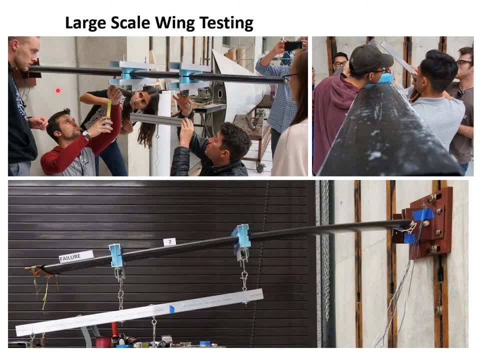 and then the important part of the and then the important part of the class as well is getting into the class as well. is getting into the class as well is getting into the testing phase right. so students have testing phase right. so students have testing phase right. so students have designed and analyzed and predicted the. 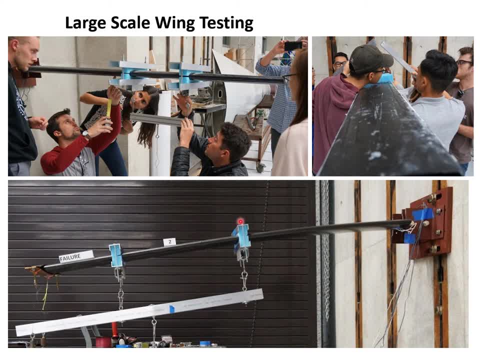 designed and analyzed and predicted the designed and analyzed and predicted the behavior we. we set this up in the lab. we behavior we- we set this up in the lab. we test it at various levels of load and behavior we- we set this up in the lab, we test it at various levels of load and. 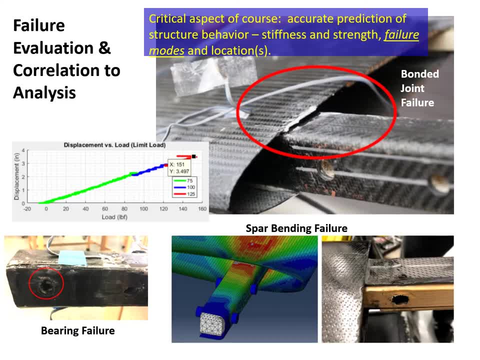 behavior. we, we set this up in the lab, we test it at various levels of load and including up to failure. and finally, the very key part of the and finally, the very key part of the and finally, the very key part of the class is comparing our analysis to the. 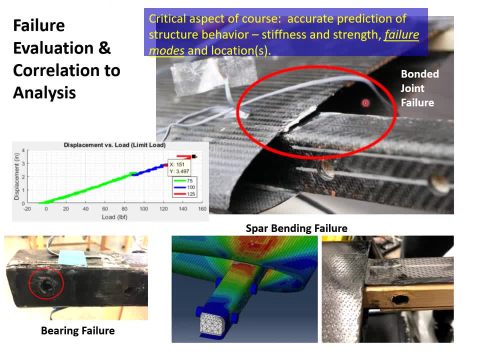 class is comparing our analysis to. the class is comparing our analysis to the failure or to the behavior that was failure, or to the behavior that was failure, or to the behavior that was experimentally measured, and so you know experimentally measured, and so you know experimentally measured and so you know this was, you know, failure. a lot of the 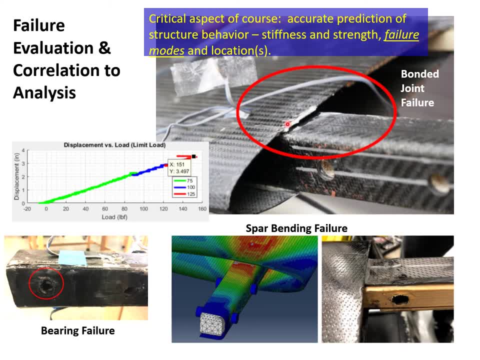 this was you know failure: a lot of the. this was you know failure: a lot of the joints are where a lot of failure occurs. joints are where a lot of failure occurs. joints are where a lot of failure occurs. can we predict that and the modeling can? can we predict that and the modeling can? 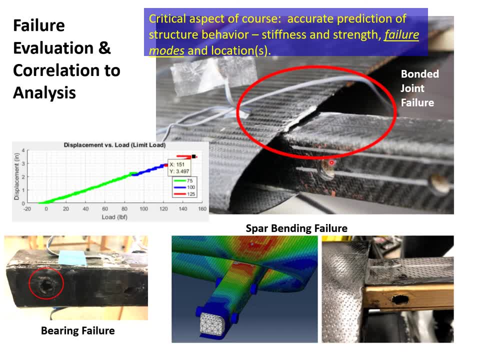 can we predict that? and the modeling can match to these predictions pretty well, match to these predictions pretty well, match to these predictions pretty well. if done right, so that just gives an idea. if done right, so that just gives an idea. if done right, so that just gives an idea about the overview of what the airspace 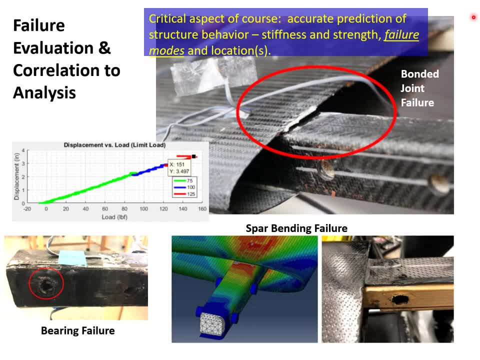 about the overview of what the airspace about, the overview of what the airspace structures focus sequence looks like. structures focus sequence looks like. structures focus sequence looks like and what you would see as an airspace and what you would see as an airspace and what you would see as an airspace: structures focus sequence- student.